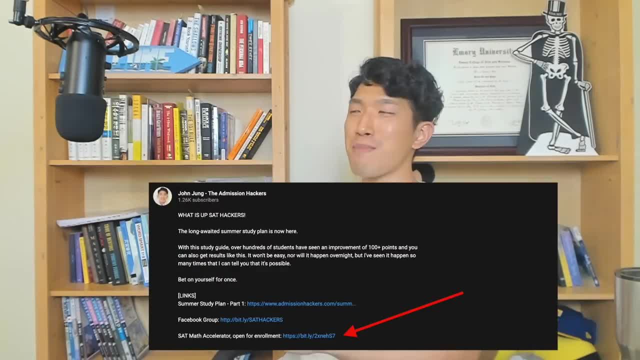 But if you're studying for the SAT right now, I highly, highly, highly recommend you check out the program, because it's the best program ever- Not because I created it, but because Sue's been getting insane results with the program. Okay, that's enough fun for the video, But the third. 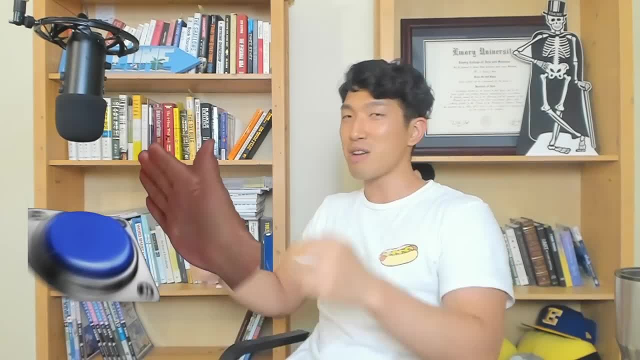 housekeeping stuff. before we get started, you guys know what to do. Smash the like button and subscribe to the channel, if you haven't already, because we will be releasing more of these. This is just part one, and there's part five, And there will be two, three, four, five. that's getting. 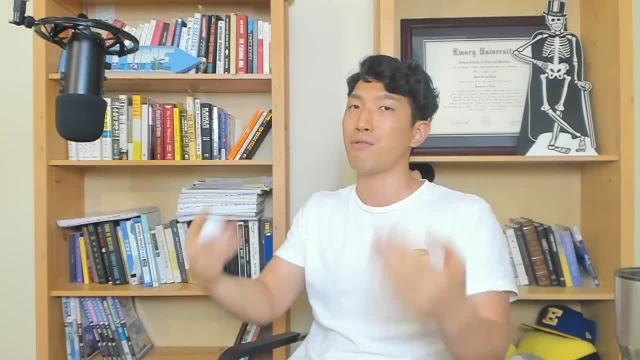 released every single week And you want to be notified when these things are available so you can take full advantage of it. So if you're ready to get started and got the cheat sheet ready, let's get straight into the video. So what do we have to know about fractions? 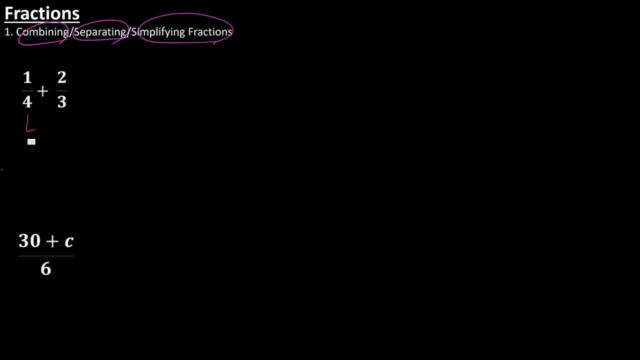 First, you want to know how to combine, separate and simplify the fractions. So when you see something like this, you want to know how to combine it into one small piece instead of having two pieces. That's what combining is, And separating when you have one piece of fraction. 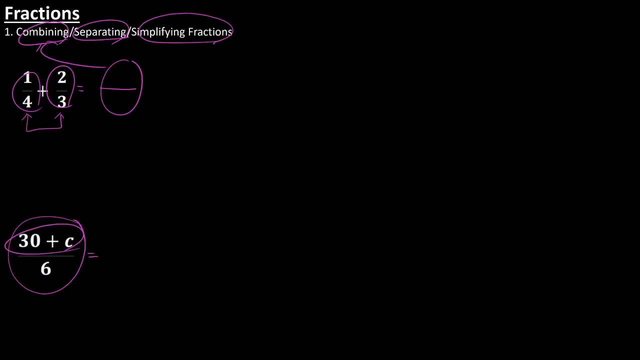 like that, but the top is two pieces like this. then you want to know how to separate it into 30 over six plus C over six. Okay, so you want to know how to combine, separate and you also want to know how to simplify fractions such as six over 18 is one third basic stuff. Next, 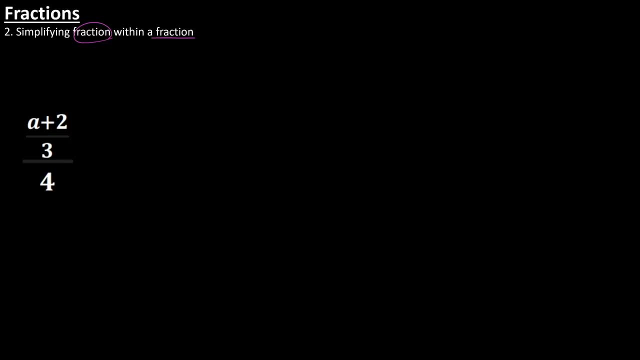 you also want to know how to simplify a fraction within a fraction. So, for instance, there is a fraction within a fraction, like that right. What we're used to seeing is something like one over four, where there's a number divided by a number. However, in this case, we have a fraction. 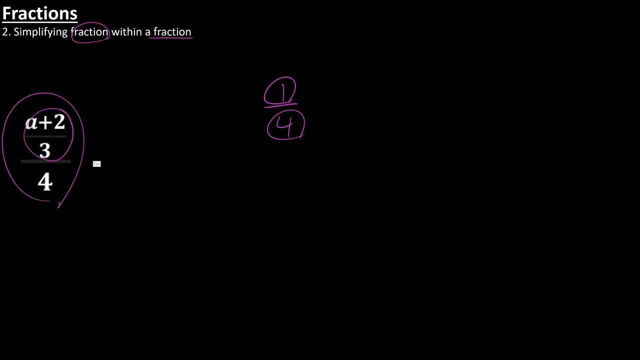 within another fraction, right? So if that's the case, you want to know how to simplify into something that looks like this: just one term over one term. Does that make sense? Next, you also want to know how to flip a fraction. So, for instance, if the question tells you that A over two is equal, 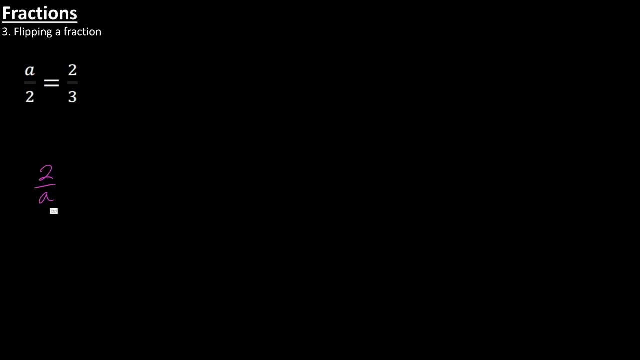 to two over three, and if it's asking you to find out what two over A is, then a lot of people find out what A is and plug it in here. But the thing is, you can actually flip fractions, And that is when you have a fraction equal to a fraction like that. then you can just simply. 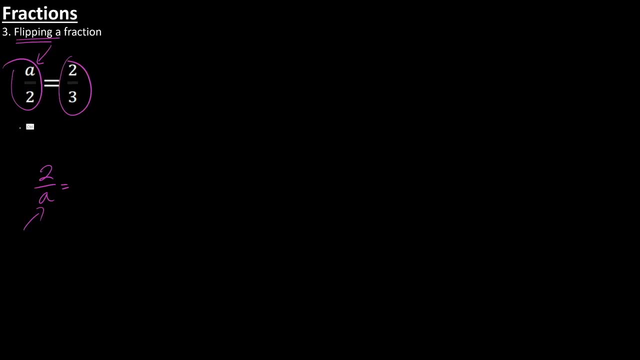 flip this side and also flip this side. So, for instance, it would look like two over A is equal to three over two. You're essentially taking a reciprocal of both sides. That way you don't have to go through all the ways to find out what A is and you just know what two over A is equal. 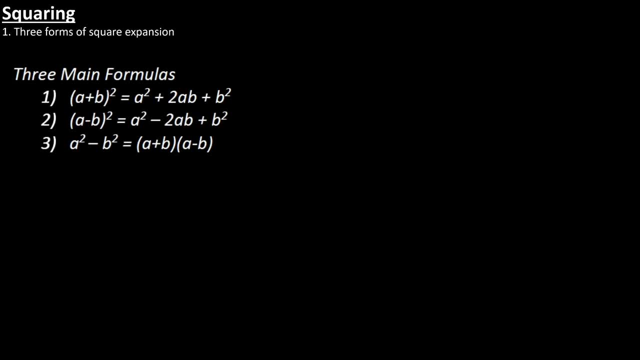 to which is three over two Make sense. It's a very important tip. Next, when it comes to squaring, there are three forms of square expansions you need to know. So the first one is going to be A plus B square, which comes out like this: A minus B square. comes out like that: A square minus B. 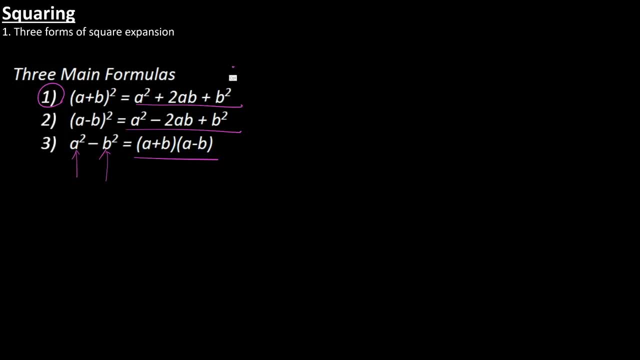 square, which is A perfect square minus A perfect square, You get the structure. You want to have these three things in your head, because they will either give you this form and ask you to convert it to that, or give you this form and convert it into that. The next type is going to be simplifying. 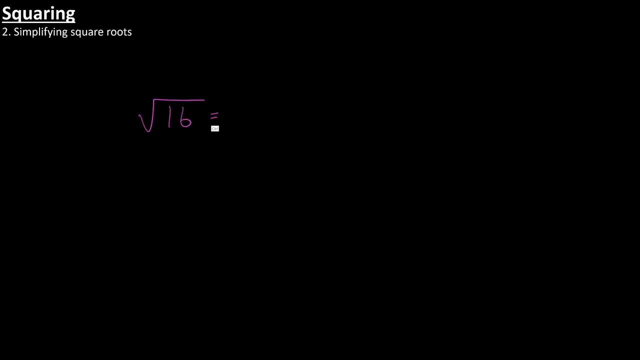 square roots. So, for instance, if you have something like square root of 16, then you want to know how to simplify this square root. For instance, it would be four. If it's a square root of 12, it would be two root three. You want to know how I got. 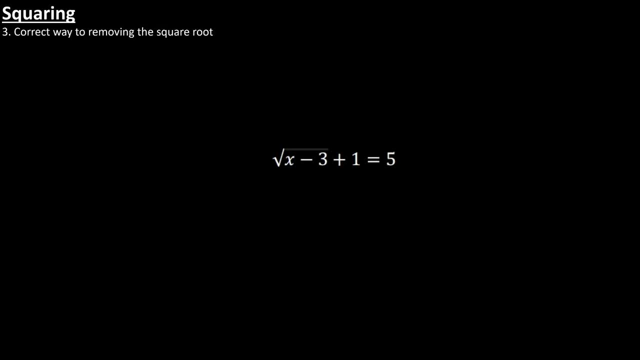 these, And if you don't, you're going to have a trouble on the math section. Next, you want to know the correct way to remove the square root. So, for instance, if you have a square root like that right there and you want to find out what X is, then you need to get rid of the square root. 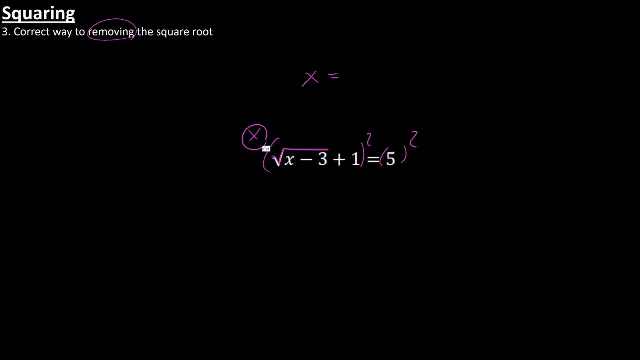 And what most people end up doing is they just square both sides like that, And that is the wrong way to do it And that is the long way to do it, Because if it's like this, you're going to have to do this twice, which becomes X minus three plus one and square root of X minus three plus one. 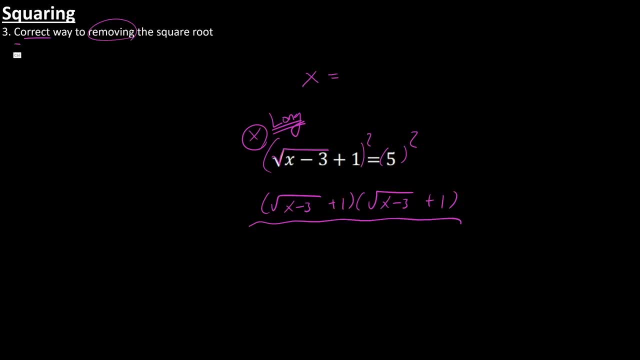 And just by looking at that, that looks really complicated. If you are doing it the correct way, then you will. you will be able to avoid this and just get rid of the, the square root, simply. Next, when it comes to advanced algebra techniques, 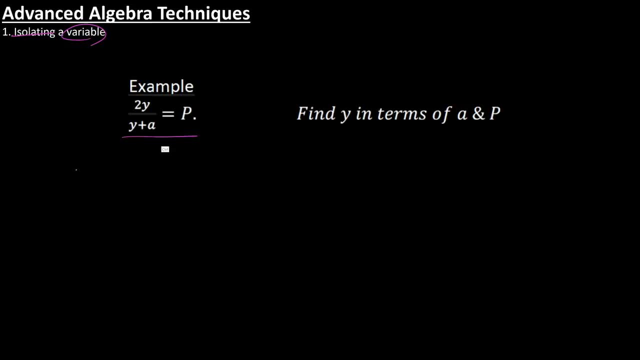 you want to know how to isolate a variable. For instance, if the equation gives you something like that and the question says: find Y in terms of A and P, all that means is: set it equal to Y. find out what Y is. set it equal to Y In terms of A and P. what that means is on this side. 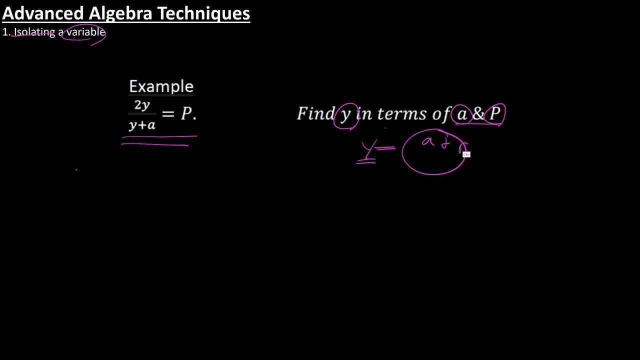 you want to have what Y is equal to, but have A and P in the equation somewhere. Does that make sense? So, for instance, Y is equal to two A over three P. you found out what Y was in terms of A and P because you have A and P as part of your answer on what Y is. Does that make sense? So for 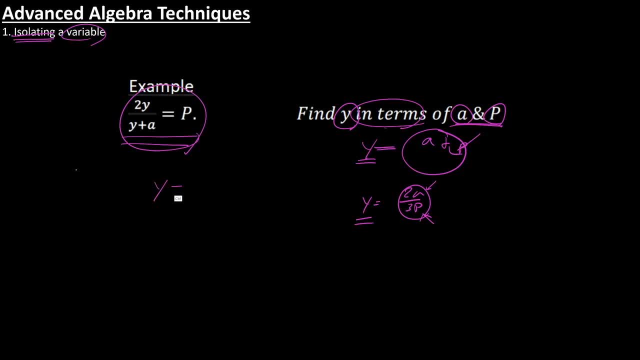 this one. you want to know how to isolate a variable so that it is set equal to Y and A and P are on the other side. Next, you want to know how to match coefficients. So, for instance, let's say we have X plus two- square is equal to this, And the question says: define the value of B right. 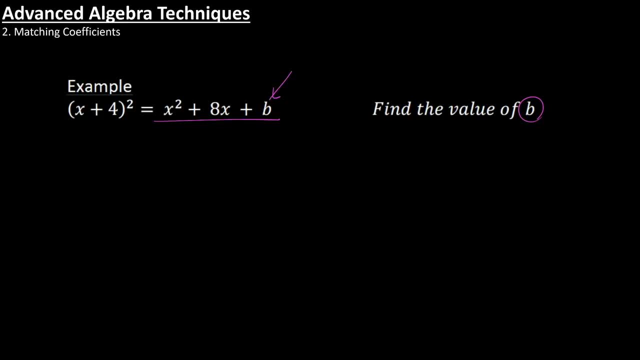 B is right there. So how would you find out what B is? It's not that complicated. So if you think about this, you know, when SAT gives you something like that, you always want to expand it. So X plus squared is going to be X squared plus eight, X plus 16.. How did I do this so quickly? Well, if 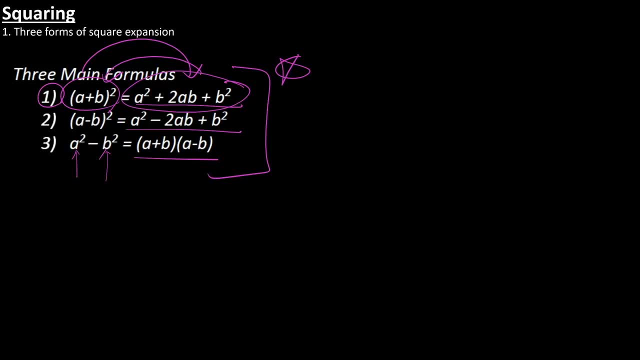 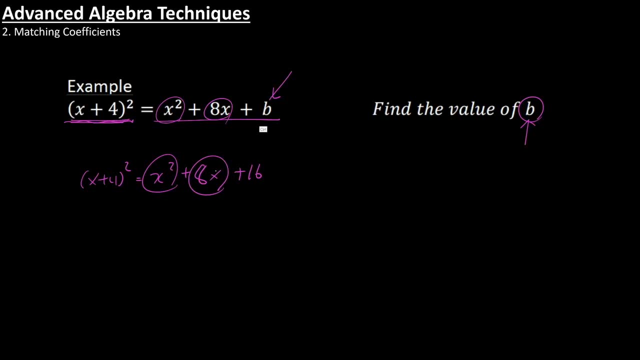 you know these three types, then you can do it that quickly. That's why you want to know these three types. But coming back to this question, the question is asking to find the value of B right? Well, if you look at it, X squared, X squared, eight X eight X B 16.. So if you 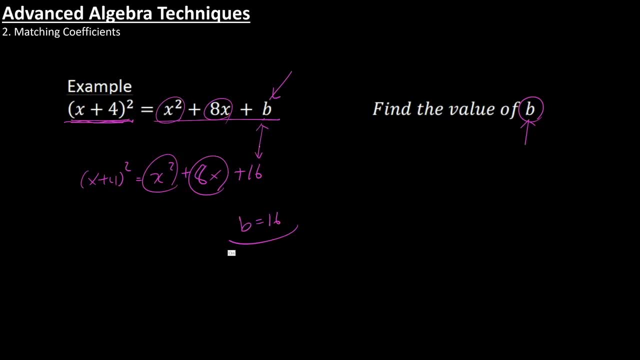 match the coefficients. if you match the numbers, you get that B is equal to 16.. And this is an important skill you need to know for the SAT, Very useful Also. you want to know how to clear the denominators. So, for instance, if you see an example like that and the question is asking you, 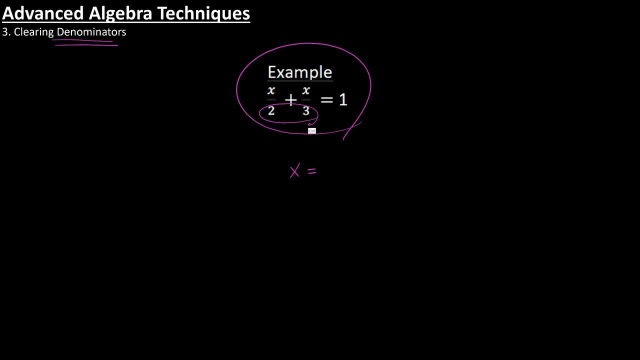 find out what X is. well, you want to know how you can get rid of T's, two and threes, the denominators, and find out what X is. You want to know how to do that And you also want to know that you can treat the complicated expressions as a whole. So, for instance, we have a complicated 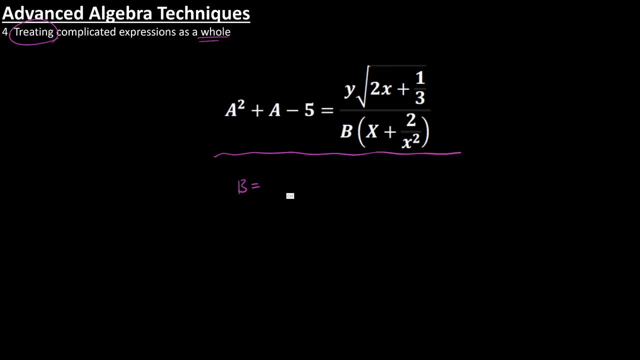 expression like that And the question is asking us to find out what B is equal to right. So if we want to find out what B is, then there's a B right there. We have to isolate the little thing right there. But the thing is that means you're going to have to multiply it by X plus two over. 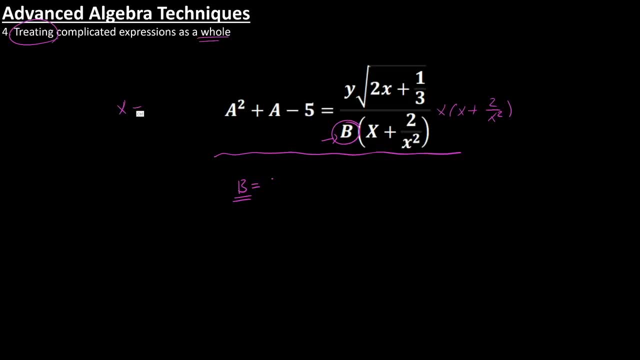 X squared And also do that on both sides. multiply it by X plus two X squared, and then we also have to like divide by that, And if you were to write everything out, it just becomes so long, right, It's just a lot of writing and that is unnecessary. So, when it comes to 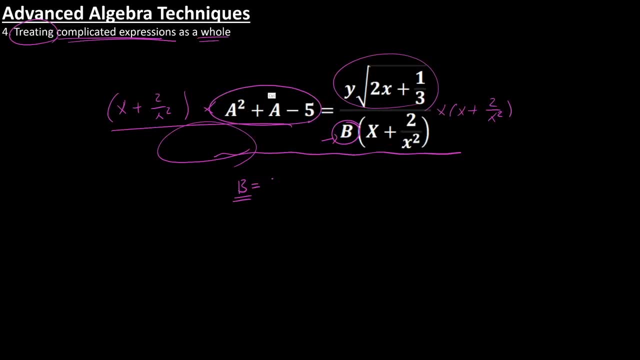 complicated expressions like this. here's what you do. See, we can just call this thing- I don't know- D, and we call this whole thing E, and we call this thing F, right, So what happens is we can simplify this equation into: D is equal to E over B, F. Does that make sense? And when you're? 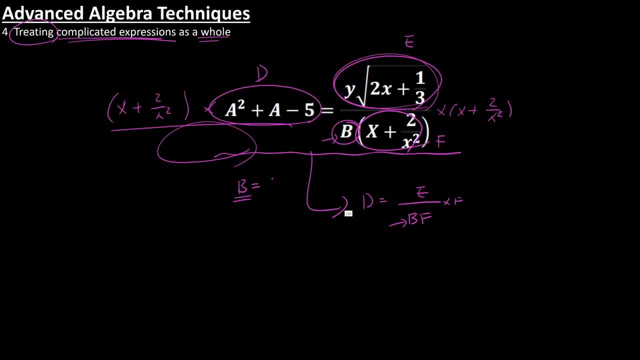 trying to isolate B. you just do the same thing. You just multiply it by F, multiply it by F and you get F. D is equal to E over B, And the benefit of doing this is that you don't have to write every single one of these pieces out. You can just write F. you can write F and you can. 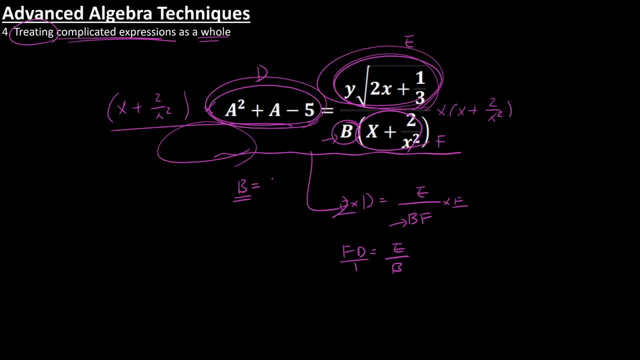 just get where you need to without writing a whole lot. And what do we do from here? Well, this is technically fraction equal to fraction, so we can flip it, which means it's going to be B over E is equal to one over F, D right, And we're looking for B, so we just multiply it by E. 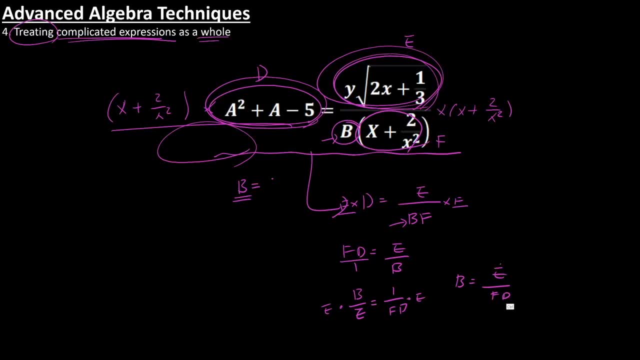 multiply it by E, we get: B is equal to E over F, D right. And after we got this, what do we do? Well, you just bring E back in here and F back down there and bring D back down there. So instead of having to write it down, 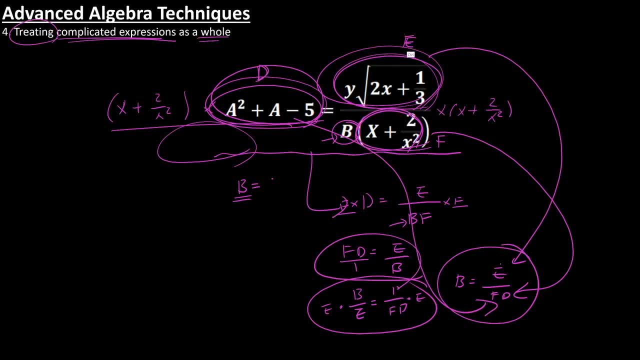 every single step of the way. you can just use simple letters like D, E and F and keep it simple, And when you actually need to, you just write it down once instead of writing it down like 10 times. That will save you a lot of time, okay, So treat complicated expressions as a whole. 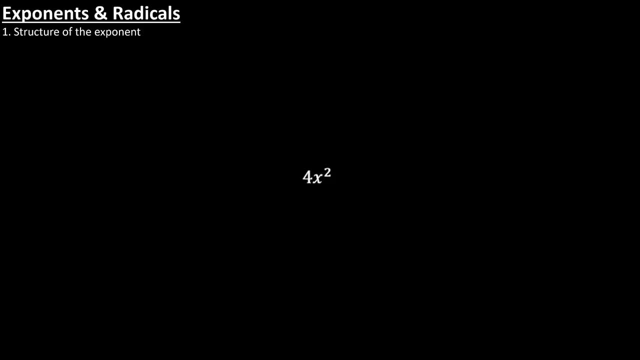 Next, when it comes to exponents and radicals, there are a lot of things you need to know, but let's break them down. First, you want to know the structure of the exponent. So what do I mean by that? Well, see this: four right there. We call this the coefficient. we call this X the base. 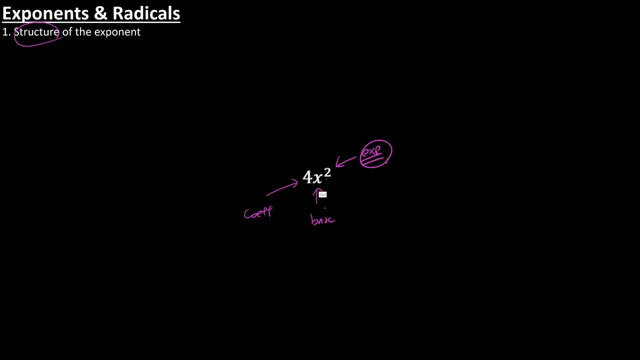 and we call this 2 the exponent right. This is the toughest part. So, if you look at it, X is called the base and not the whole 4X, because 2 is only applied to the X right. It's not applied. 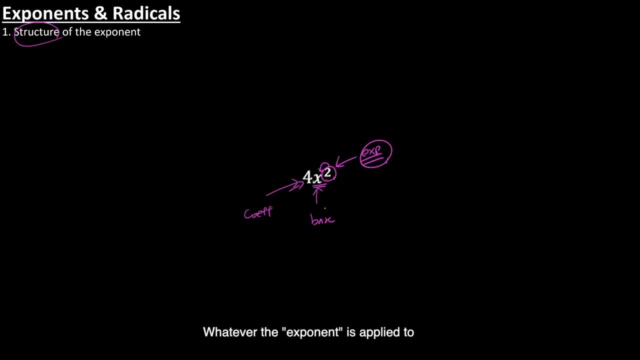 to the 4, it's only applied to the X, And whatever the base is applied to, that's what we call the base. Does that make sense? So you want to know the difference between that and that? okay, In this case, 2 is applied to both 4 and X, so 4X is known as the base. However, in this case, 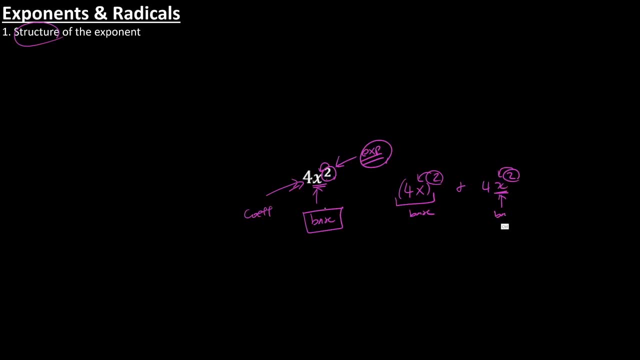 X is the only thing that's applied by the 2, so we call it the exponent. So what do we do? We call X the base. okay, You want to know the difference between the two. You also want to know how the 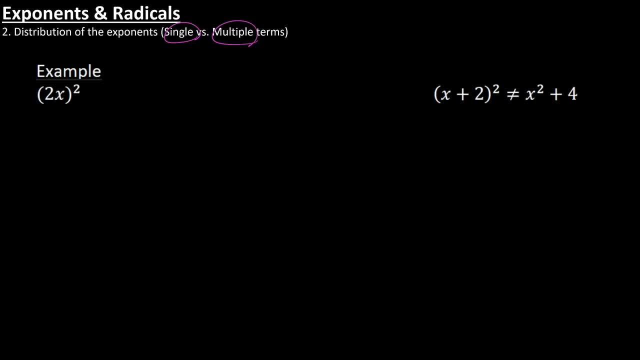 distribution of exponents work. So, when it comes to single term versus multiple terms, what do I mean by that? Well, when you see 2X squared and you see X plus 2 squared, you don't do it the same way. This one, you would distribute the exponents, but this one, you would have to. 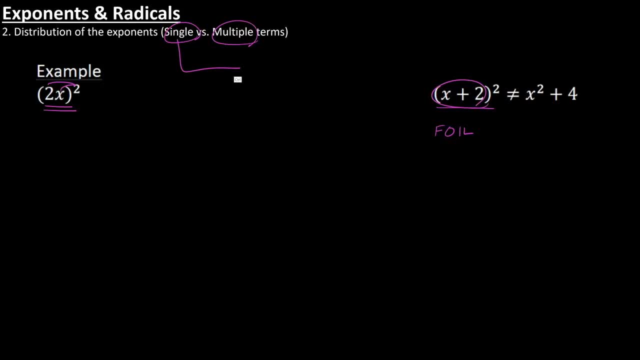 FOIL, And that's because it has multiple terms. okay, You want to know the difference between the two. This is a very common mistake a lot of students make, because when they see that a good chunk of the students do what they do is they just do this, which becomes X squared plus 4.. 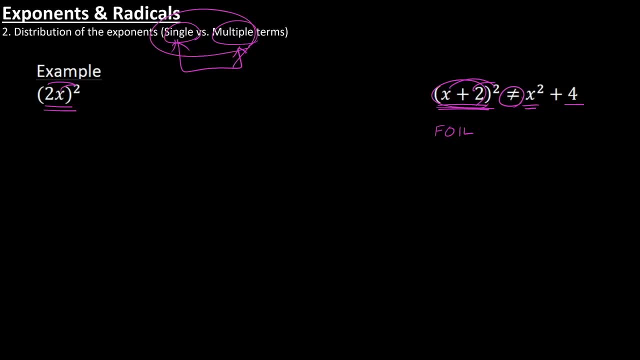 And that's not true. That's not right. okay, You want to know the difference between the two. Next, you also want to know how to convert negative exponents to positive exponents. So when you see that SAT, you cannot have negative exponents in your answer, So you have to find a. 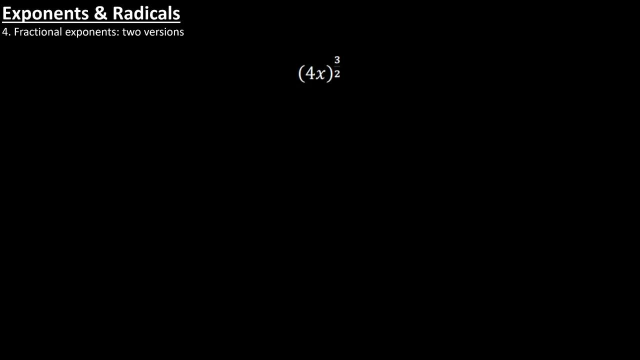 way to get rid of this negative exponent into a positive exponent. Does that make sense? Cool. So you also want to know how fractional exponents work. So what we're used to seeing is just regular good old exponents like that, but sometimes you will see a fractional exponent right Then when. 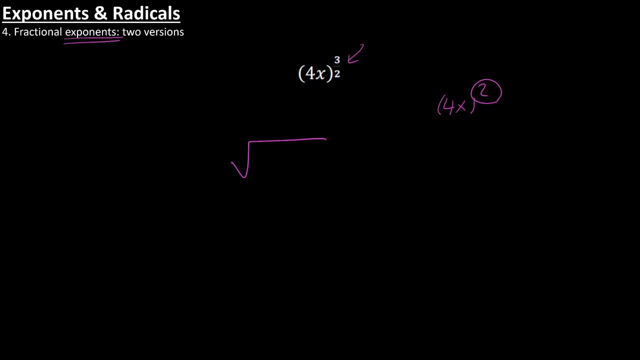 it comes to fractional exponent, they go inside a radical. okay, So this one will be 4X: whole thing square or cubed Over square root. It can look like that, or there's going to be other version, but you want. 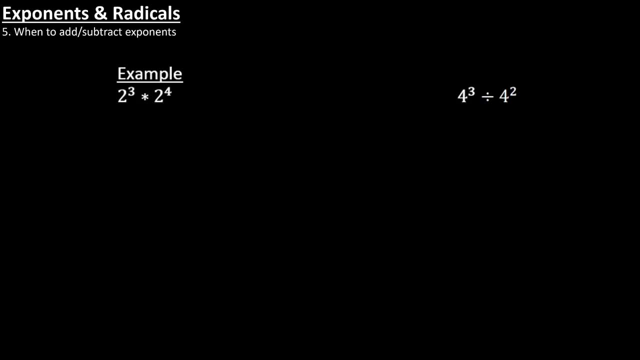 to know both ways. Does that make sense, Cool? Next one: you also want to know when to add or subtract exponents. So, for instance, when it comes to 2 to the 3rd times, 2 to the 4th, we know that. 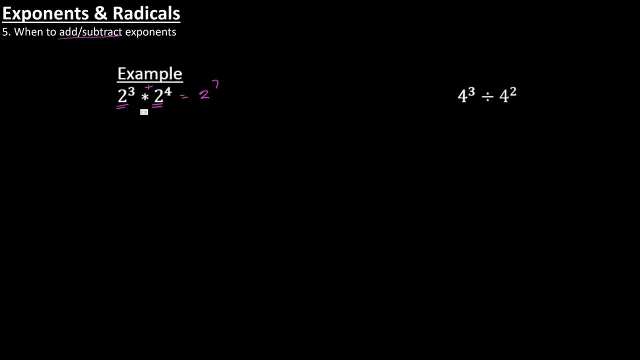 it's going to be 2 to the 7th. You can add the exponents when your bases are the same and you're multiplying that, which becomes 2 to the 7th, And when it comes to 4 to the 3rd, divide by 4 to the. 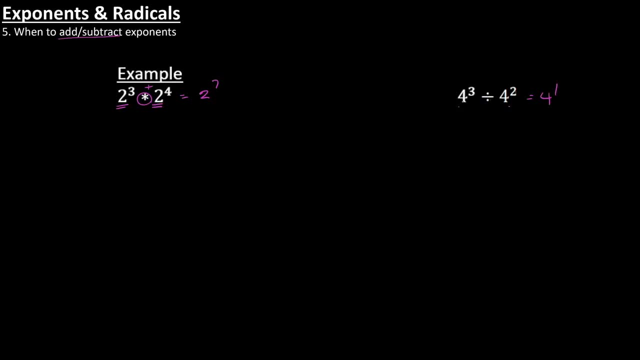 2nd, When you're dividing same base, what you do is you subtract the exponents. Next one: Also, you want to know how to multiply the exponents. It's important to know when to add and subtract exponents, but also when to multiply. 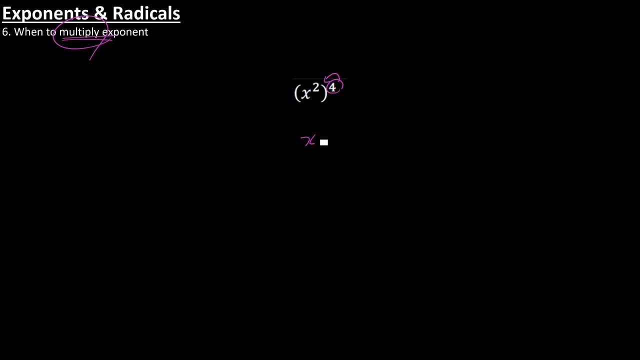 So in this case, when there's an exponent on top of an exponent, that's when you multiply the exponents. Also, you want to know how to match the bases. So, for instance, 9 to the 2nd divided by 27. 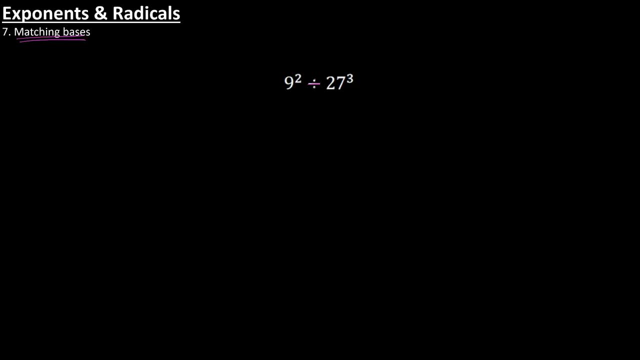 to the 3rd right. So when there's an exponent and when we're dividing, we would usually subtract the exponents right. But the thing is we can't subtract the exponents because your bases are different. Remember, when you're adding or subtracting exponents you have to make sure 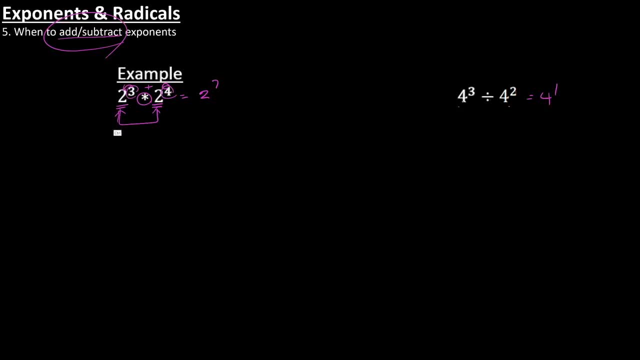 that your bases, or whatever the exponent is applied to. we have to make sure that the bases are the same. That's the only time you can add or subtract the exponents, But in this case the bases are different. So when you're adding or subtracting exponents, you have to make sure that. 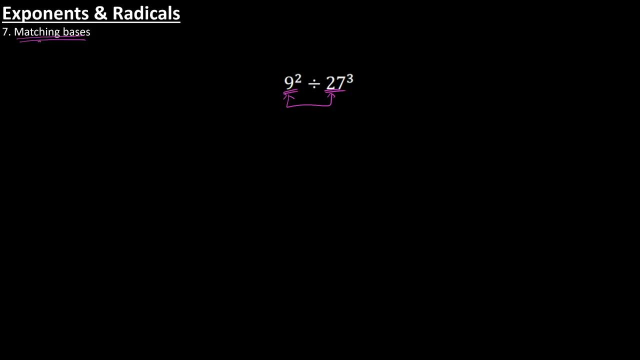 So you want to know, you want to find out a way to match the bases so you can work your exponents and get the answer. Another thing is that you can actually also pull out exponents. So what do I mean by that? Well, let's look at this question right here: 2 to the x plus 3 is equal to 2 to 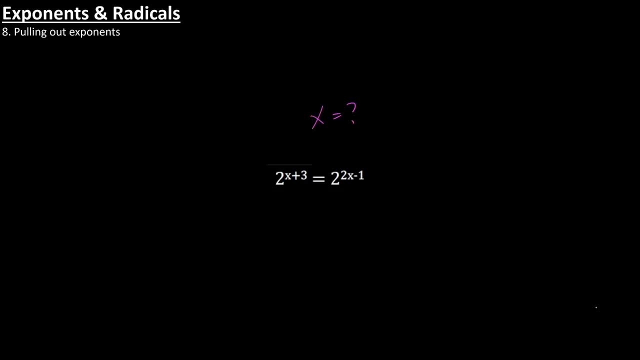 the 2x plus 1.. And if the question is asking you to find out what x is, it's a tough question. because if it were just like, x plus 3 is equal to 2x plus 1, then you can just move stuff around. 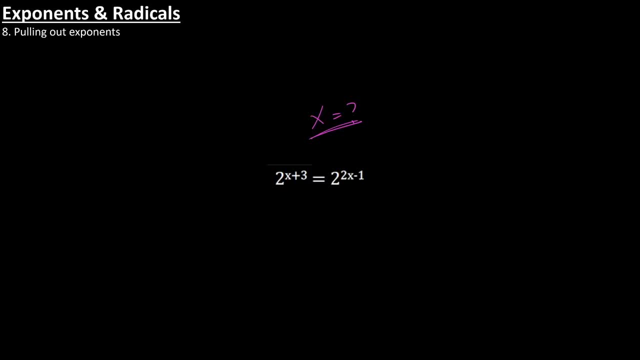 easily and find out what x is. But it's hard because x is now used as an exponent. But here's the thing: You can actually pull these out and just write down: x plus 3 is equal to 2x minus 1.. 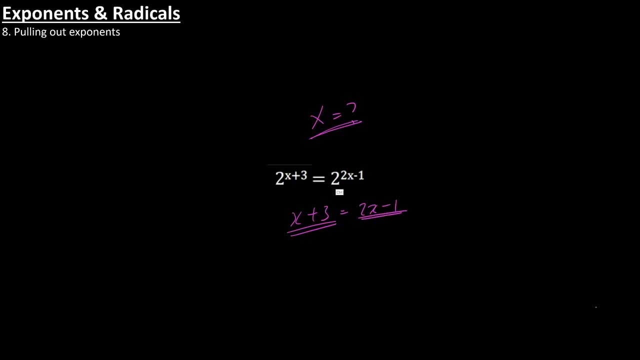 And then you can just move stuff around easily and find out what x is. But here's the thing You can do. that is because as long as your exponents are equal to each other, your whole thing will be equal to each other, right? Because when exponents are the same, then your results will be the same. So 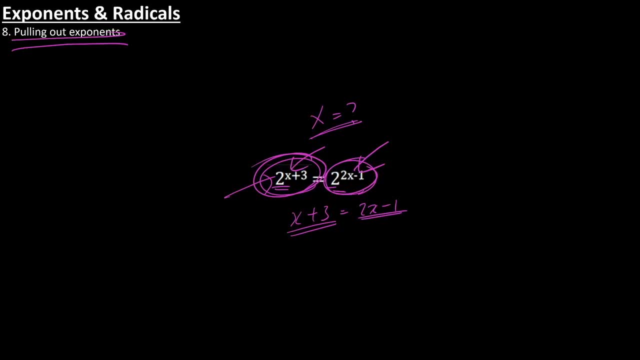 you want to know that you can pull out exponents when the bases are the same. Does that make sense? Cool, Let's go to the next one. So simplifying radicals. So we knew how to simplify, like square root of 18.. But what about variables like this? You also want to know how to simplify this, and 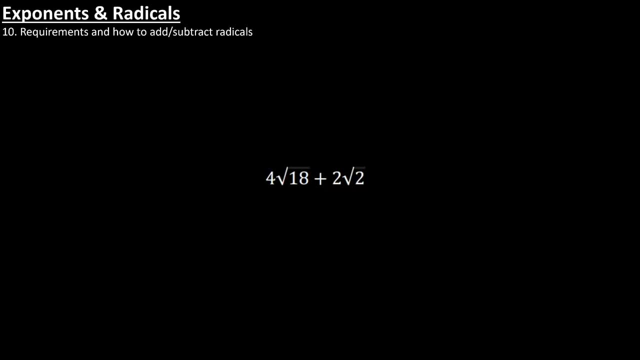 it would be x cubed x. Next one: requirements and how to add, subtract- radicals right. So when it comes to radicals, there's two things you need to know. You want to know how to multiply and divide and add and subtract. So, when it comes to addition and subtraction, can you do this? No, 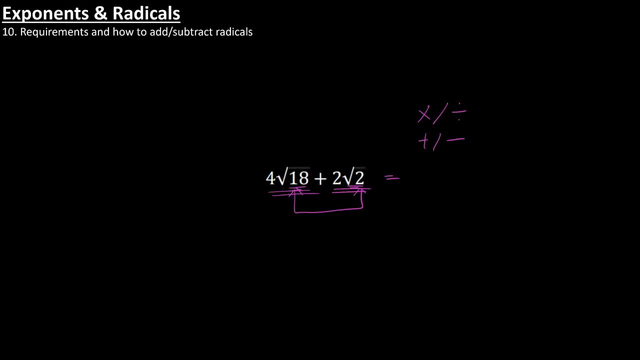 you can't See, in order for you to add or subtract, radicals, the insides have to be the same, but they don't. So that's the requirement. you want to simplify and you want to know how to add and subtract. When it comes to multiplying, well, when you're multiplying, there's no. 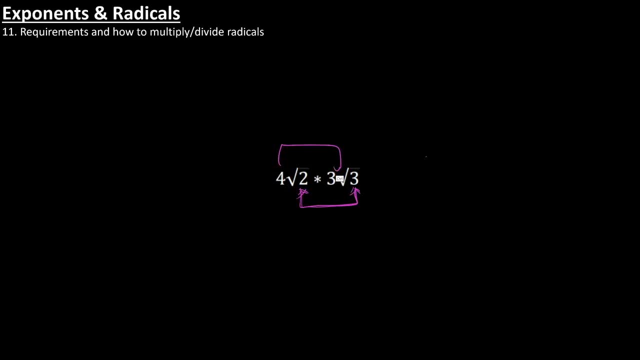 requirement. What you do is you just multiply the inside of the radicals and outsides of the radicals together, So it will become 4 times 3, which is 12 square root of 3 times 3, 6.. Does that make sense? So, addition and subtraction. there is going to be a requirement, which is 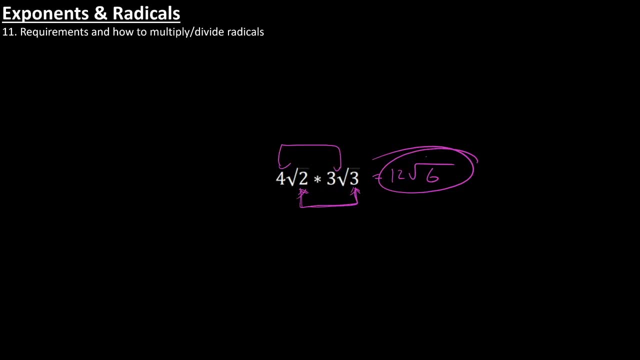 the same. So you want to know how to add and subtract. So when it comes to addition and subtraction, inside, but when it comes to multiplication or division there's no requirement. You just do inside, inside, outside, outside And the percent chapter. So first, when it comes to percent, 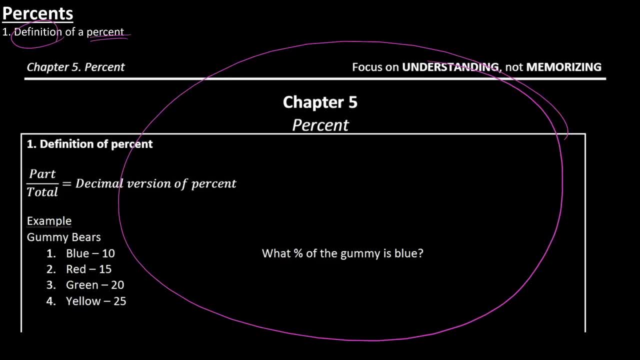 you want to understand the definition of percent. So this is like a little worksheet that we do in SAT Math Accelerator, but it's like an example, So I just pulled it out for you guys. So, percent chapter: Well, first you want to know the definition of percent, and the definition is: 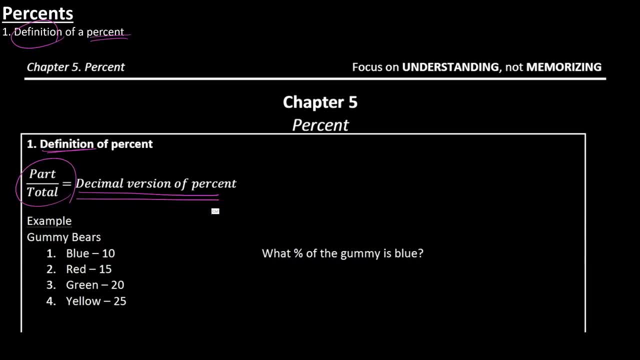 part over total. Okay, Part over total will give you the decimal version of the percent, And you might be thinking: what the heck does that mean? Let's think about it. So the question says: what percent of the gummy bear is blue? right, We want to find out the percent of. 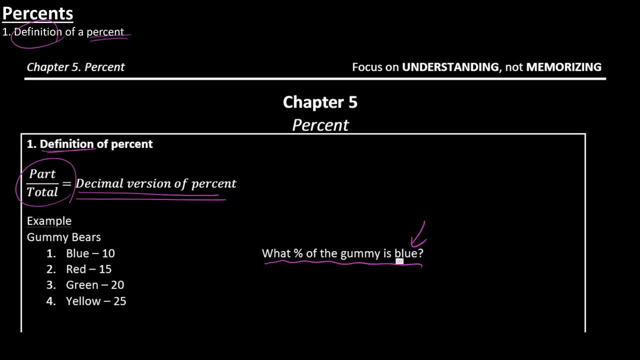 blue gummy bears, right. So how do you find percent of blue gummy bears? You do part over total. Okay, What you do is you do number of blue, which is the part of the whole thing, and you divide it by the total. So if you look at these numbers right here: 10 blue, 15,, 20,. 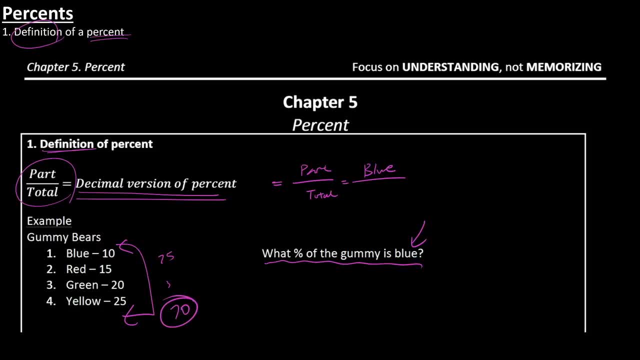 25 yellow ones. So if you add them all up- 25,, 50,- you get 70. So your total is going to be 70, right? So how many blues do you have? You have 10.. That means one over seven or 10 over 70,. 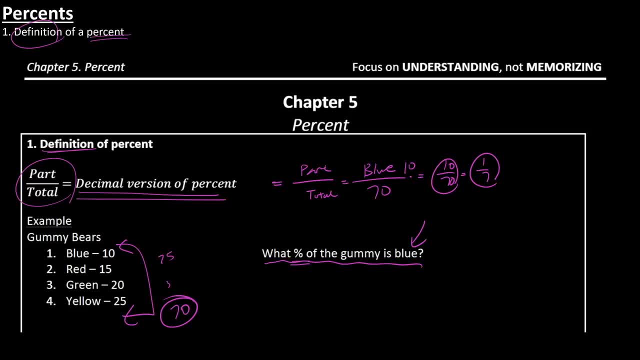 which becomes one over seven. That is going to give you the percent, And if you divide it you're going to get 0.14.. One divided by seven gives you this right. So 0.1428 is going to be the decimal version of. 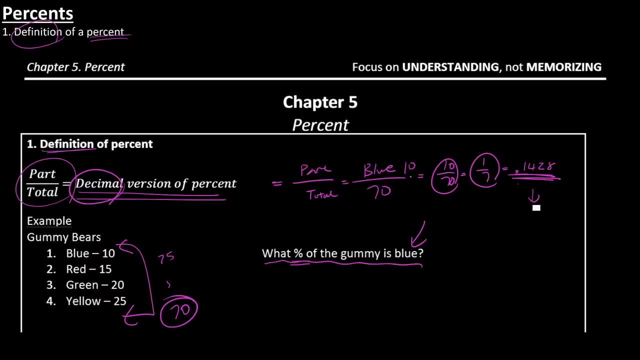 the percent. Okay. So how do you convert decimal version into a percent version? Well, you just move two decimals to the right. So 0.1428 is equal to 14.28%. Okay, So that's just the decimal version. That's going to be a percent version. Okay, But when you do part over total, it gives 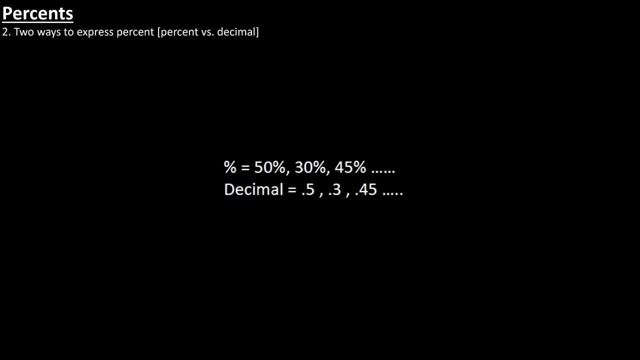 you the decimal version And when it comes to percent, there are two ways to express percent. Remember, there's the percent version and there's a decimal version, Just like we did here. there was a decimal version and there's the percent version. There are two ways. Okay, 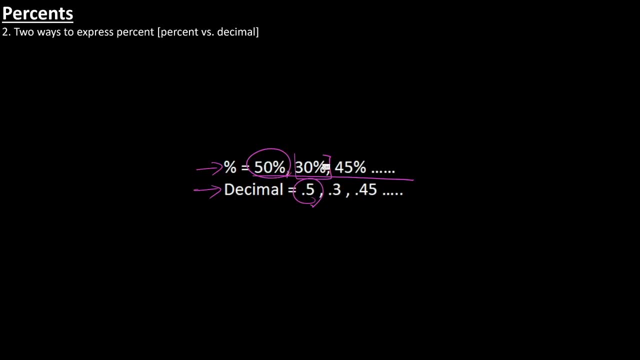 Percent version: 50% is same thing as 0.5.. 30% is same thing as 0.3 and 45% is same thing as 0.45.. Okay, Two ways to express percent. which is percent version? decimal version. You want to know both. 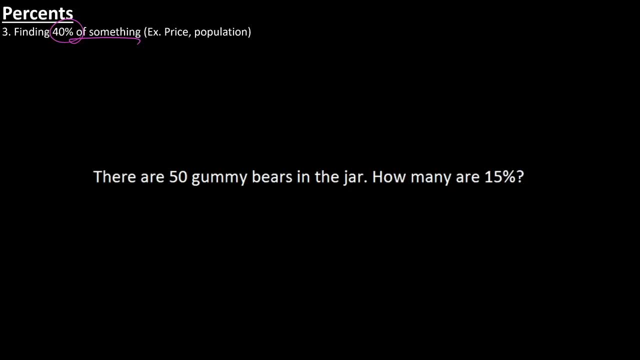 Next thing: when it comes to percent, you want to know how to find 40% of something. So, for instance, if the question says there are 50 gummy bears in the jar, how many are 15%? You want to know how. 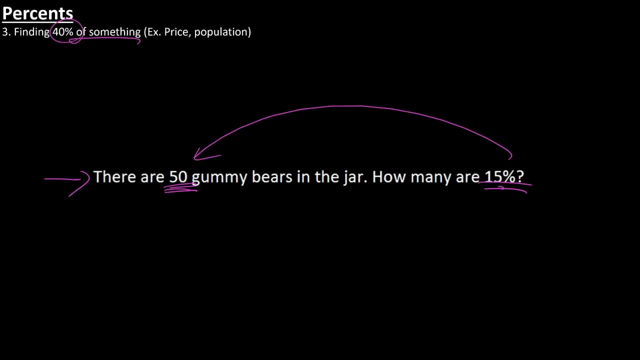 you can find 15% of 50. Okay, 15% of 50. How do you do it? That's what you want to know. It's tested on the SAT. Second, the question will also say finding. how do you find 40% decrease of something right? So there's a difference between finding 40%. 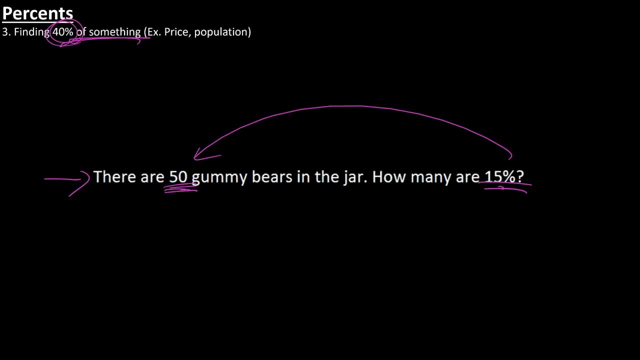 decrease of something versus finding 40% of something. For the first one you're just finding 40% of something, Whereas the second one you have to find 40% decrease and find the remaining. Does that make sense? That's the difference. They will test you on both ways. 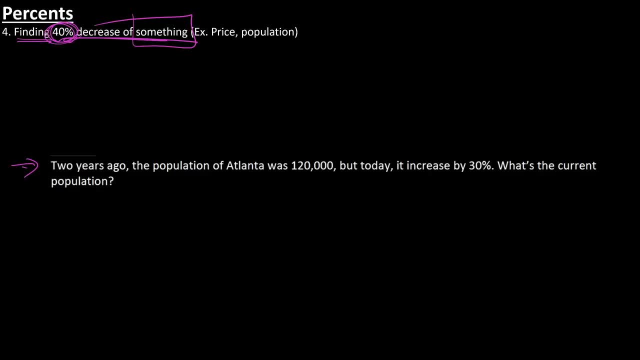 There are different things. So, for example, it's going to look something like this, which is also an example from SAT Math Accelerator, down below in the description box: So two years ago the 120,000, but today it increased by 30%. What's the current population? So it went from 120,000. 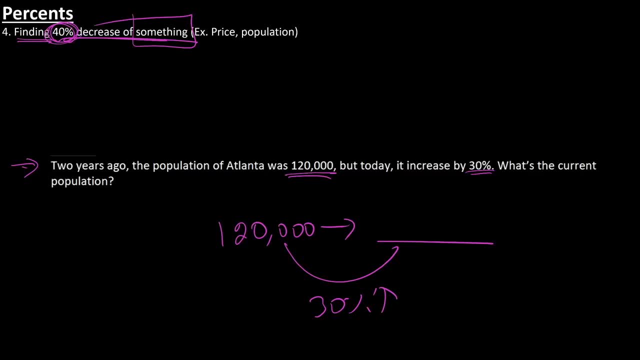 to certain and there was a 30% increase. right, You want to know how you can find 30% increase or 30% decrease of whatever. Remember it's different from 40% of something versus 40% decrease or 40% increase. Make sense. Next one: Also, you want to know how to calculate the. 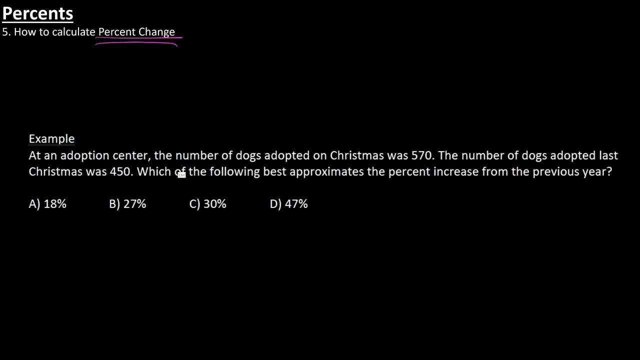 percent change. So what do I mean by that? Well, here's an example: In an adoption center, the number of dogs adopted for Christmas was 570, right? The number of dogs adopted the last Christmas was 450, right? So last Christmas, I gave you my heart. 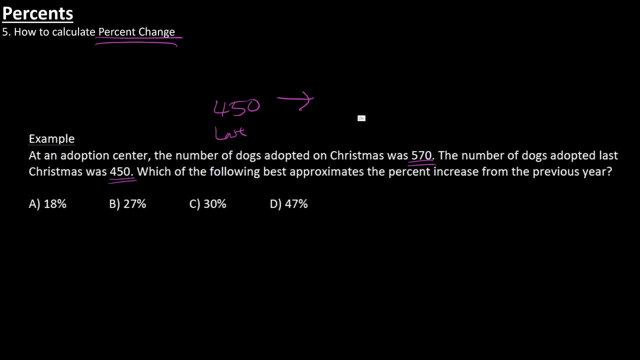 No, 450 was last year right, And then it became 570, which is this year right. So it went from 450 to 570.. And the question is asking which of the following best approximates the percent increase from previous year? You want to know what the percent increase was from 450 to 570. 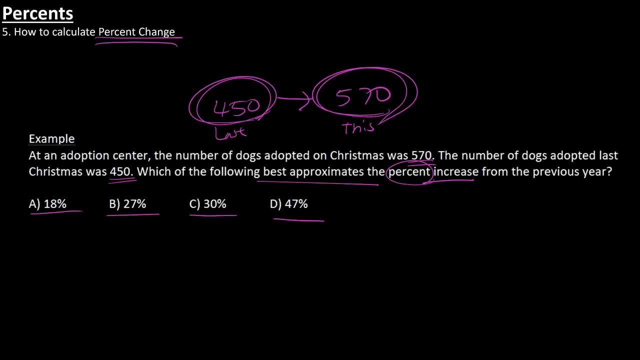 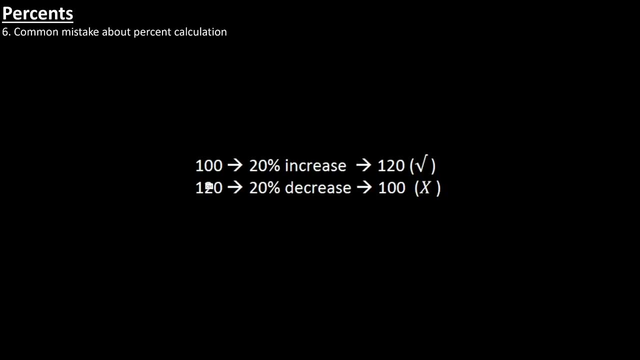 And there is a simple formula for it, but you want to know how to do that. And the last thing about percent you need to know is going to be the common mistakes that people make about percent calculation. So here's the thing: See, if you have a hundred right And if you increase it by 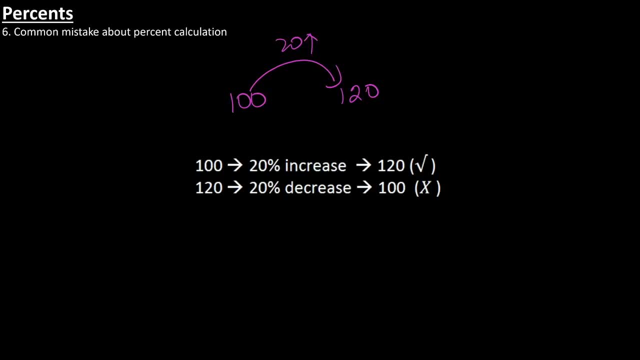 like 20%, you're going to get 120.. Okay, Let's say we increase it by 20% and then you get 120.. And if the question asks you, by what percent decrease would you need to do to go from 120? 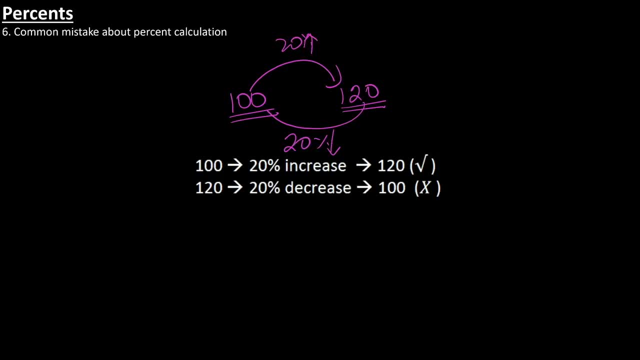 to 100?? Most people would just say 20%, because that's a logical thing, because you increased it by 20% to get 120. Then you would do the opposite, to go back to where you were before. but that's not the case. That is the common mistake that people make. So if you increase it by 20%, you 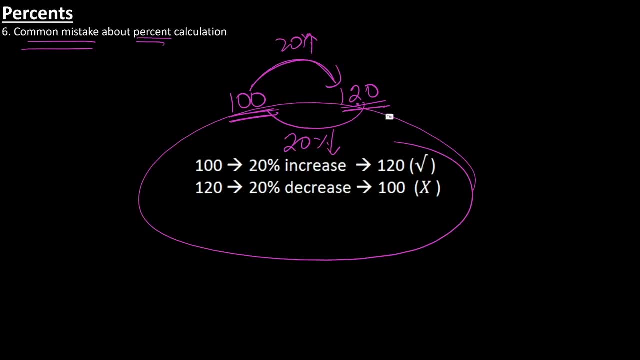 when they're doing percent calculations. So you want to know how to calculate what percent decrease you need to do in order for you to get back to 100 from 120.. So that's going to be it, guys. These are the basic things that are covered in the SAT. So, while you're studying for the SAT, 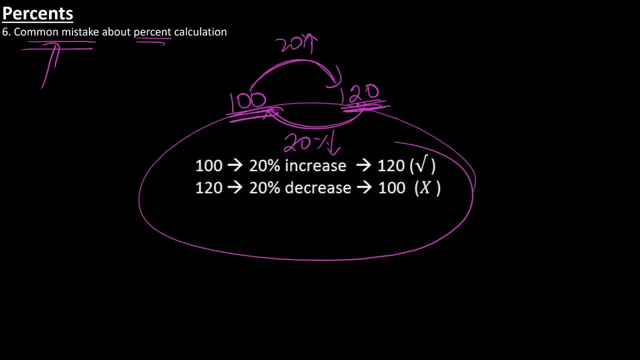 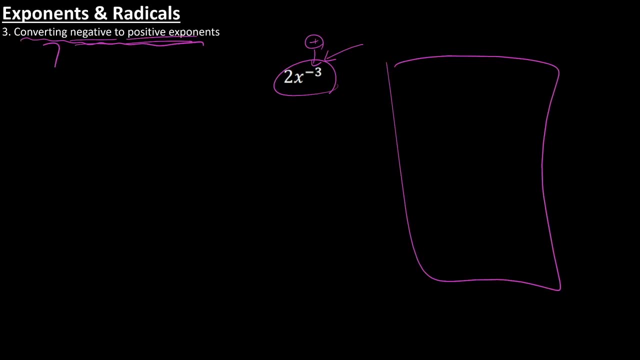 make sure you know these things. you know for percent, you want to know the common mistake And, when it comes to radicals and exponents, you want to know how to convert negative exponents into positive exponents. So you know, there's a little worksheet that you printed out: Make. 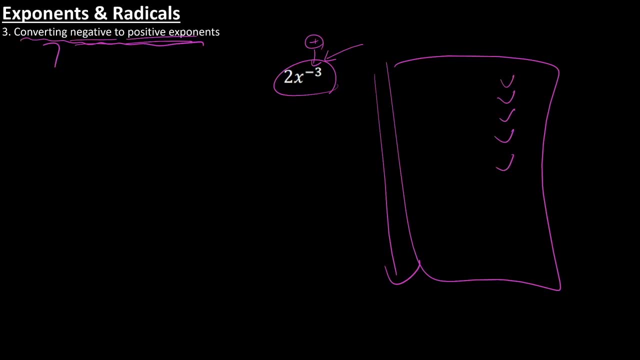 sure you go through the list and make sure you can check- I know this, I know this and I know this for every single one of these. Otherwise these things will show up and they'll bite you and you're going to lose some points and it's not fun. So if you guys have any questions or 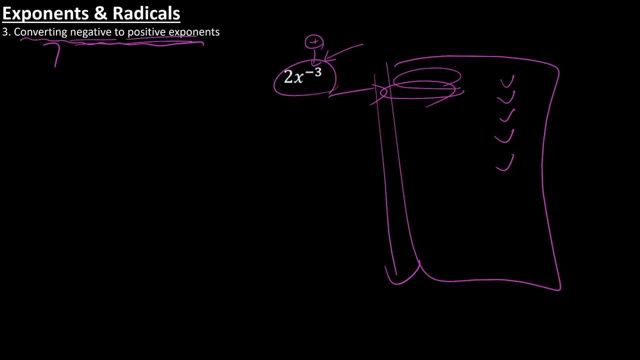 comments, leave them in the comment section down below And if you're interested in the program, check out the SAT Math Accelerator in the description box down below. And although this is just part one, there are four more parts coming dealing with word problems: geometry. 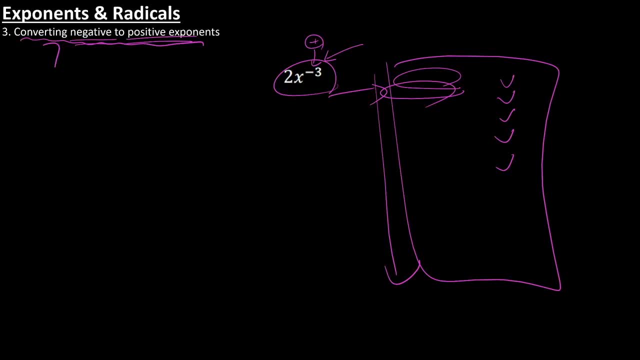 functions, advanced SAT math concepts. So if you're interested, if you're studying for the SAT right now, make sure you subscribe to the channel and turn the notification bell on so that you'll be notified when these videos are up and you can take full advantage of them. And, as always, 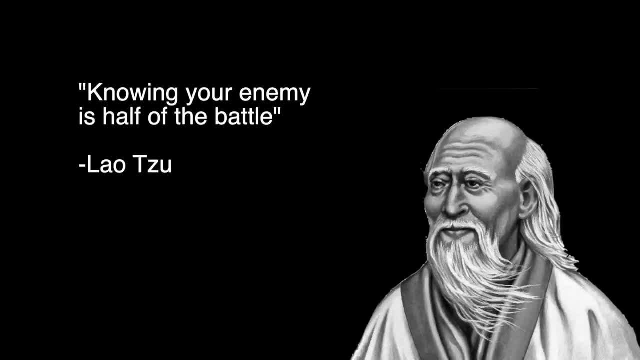 I'll see you on the next video. Bye.